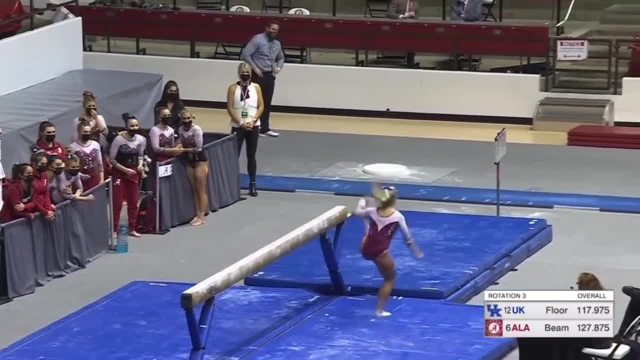 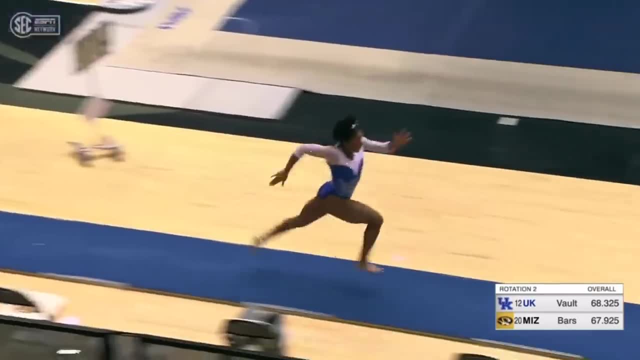 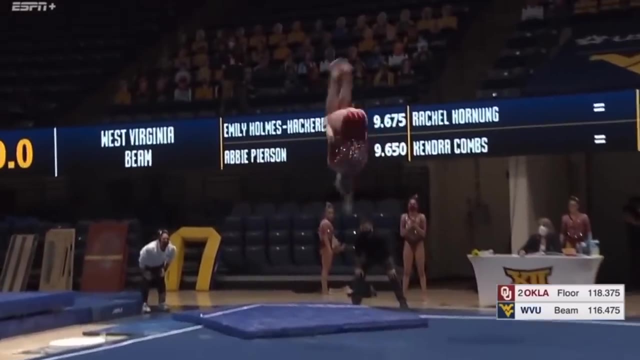 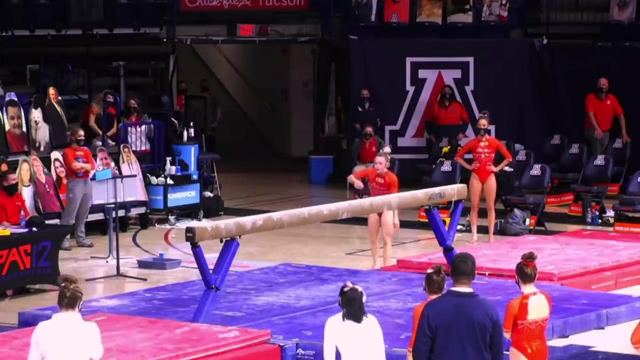 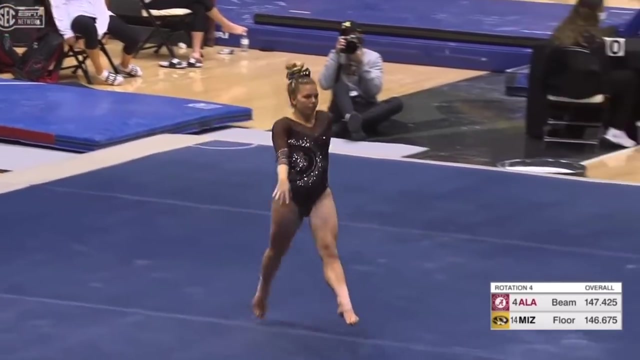 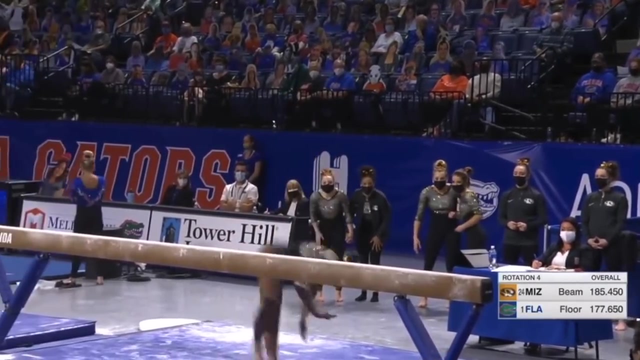 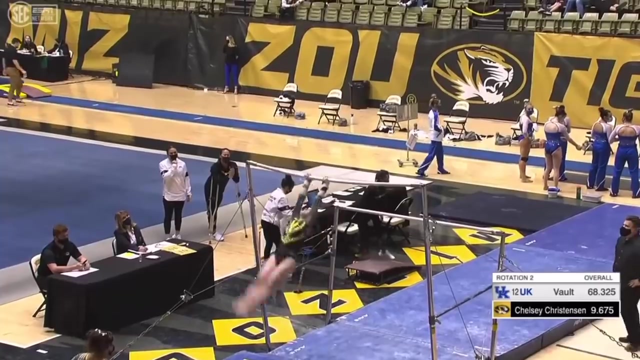 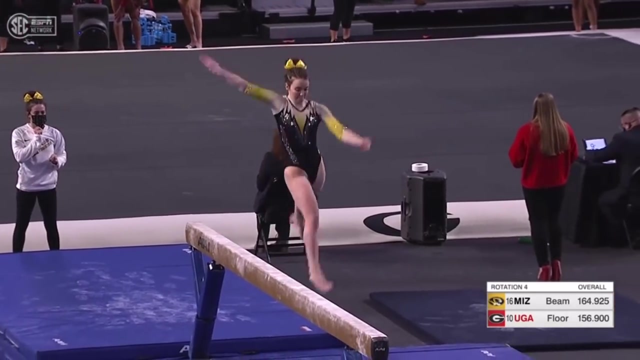 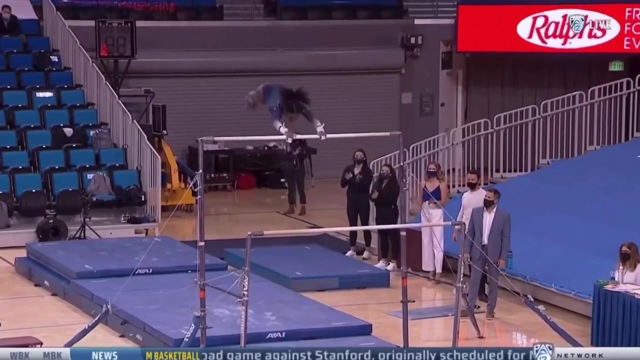 Please subscribe to our channel and hit the bell icon to get notifications of our new videos. Oh, Front aerial Battle: jaeger, Battle, jaeger. Front position. Being in this lead off position, it really sets the tone for the remainder of the bar. 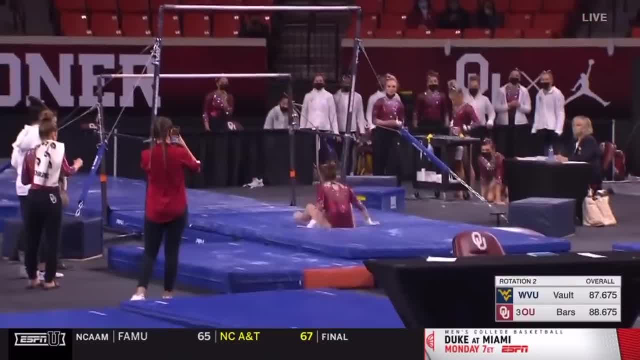 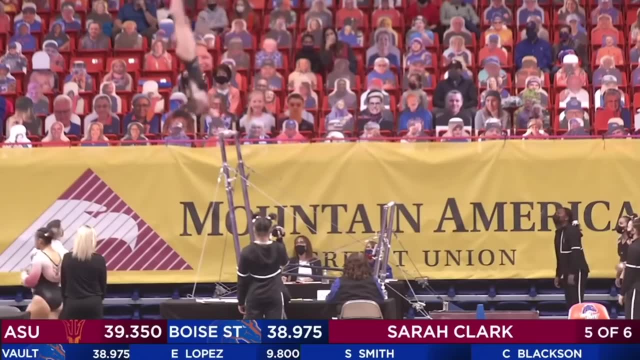 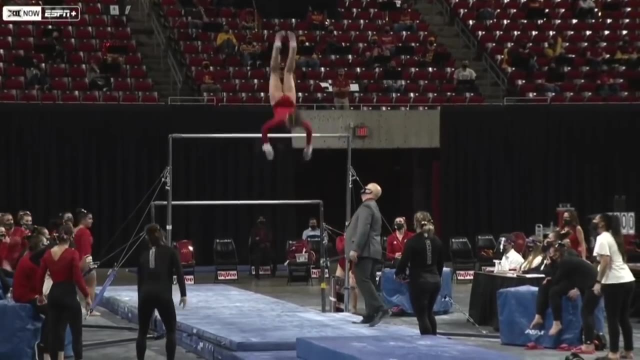 Sets up this dismount. Watch this Double front. Oh Her, Did her Stronger, take a four and a half Dismount. Another look at the dismount Which didn't go as Gomes had planned. Oh, 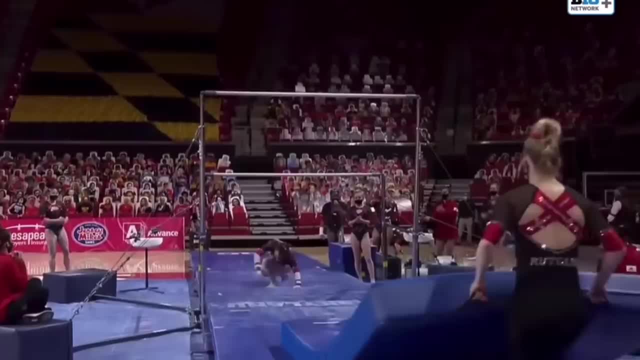 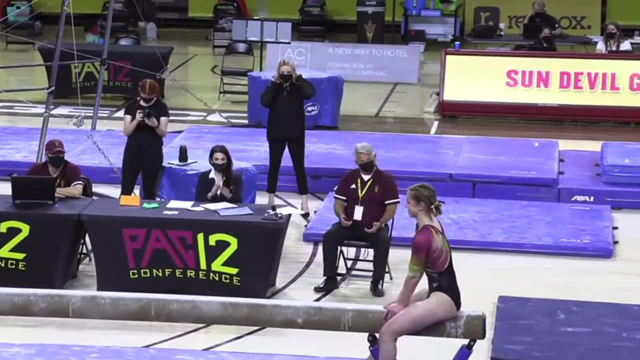 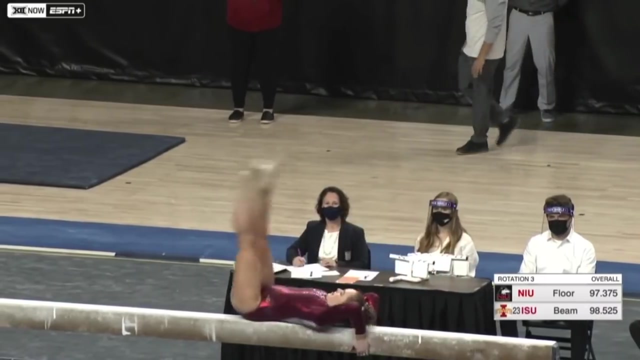 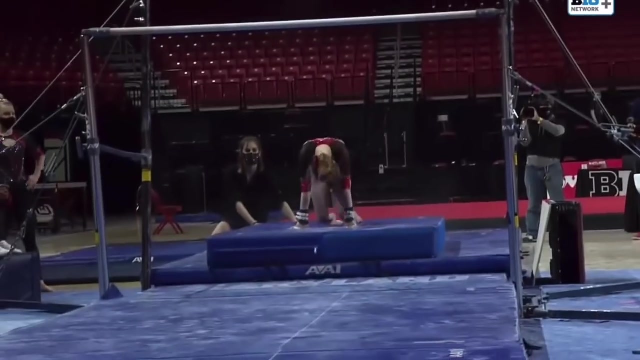 Fought for it Into a jaeger. Really difficult series right here Back handspring Layout, Layout, Oh Oh, Extra swing pretty well, And then double front dismount, Oh, Close call. See a Oh, Big release. 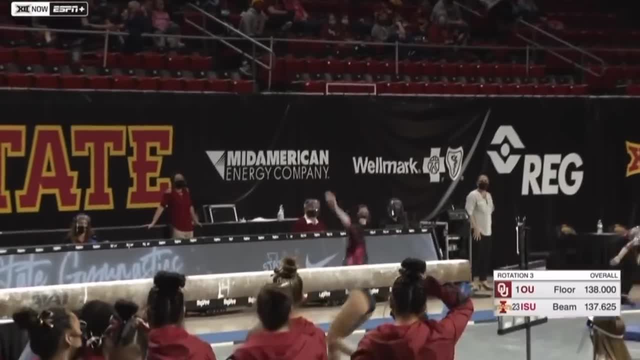 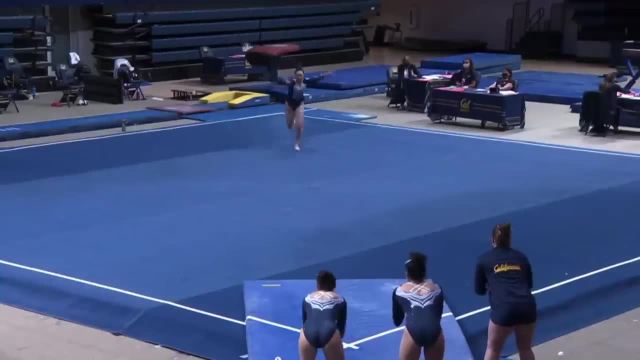 Let's look at the last set. I'm gonna have to say no to that. Not gonna do any of it. Not gonna do any of it. Yeah, Oh, my gosh, Oh, Oh, Oh, Ready, Yeah, Oh. 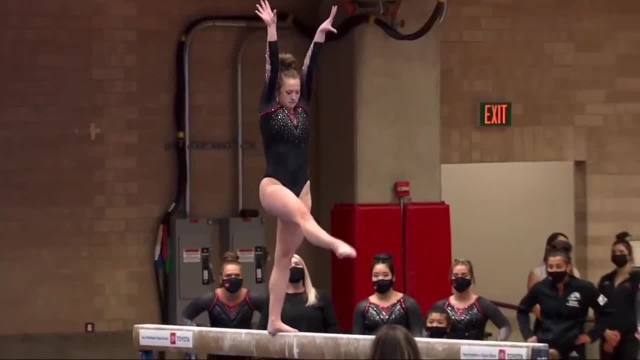 Oh, Oh, I'm so excited. I'm so excited, guys, I must say I'm so excited. She's a little bit out of breath. She's moving on her feet. She's moving on her feet. Oh my gosh.